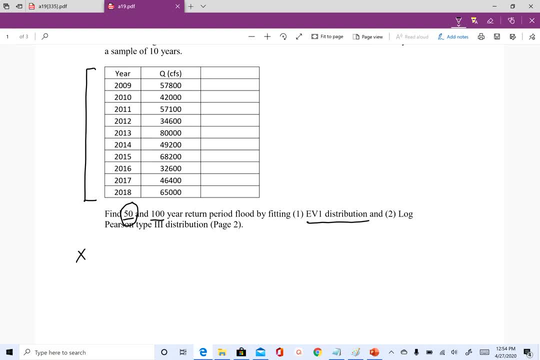 that we have for EV1 is: Xt is equal to X bar minus square root of 6 divided by pi, And then 0.5772 plus natural log of natural log of t over t minus 1, and the whole thing is multiplied by the standard deviation. Okay, so X bar here is. 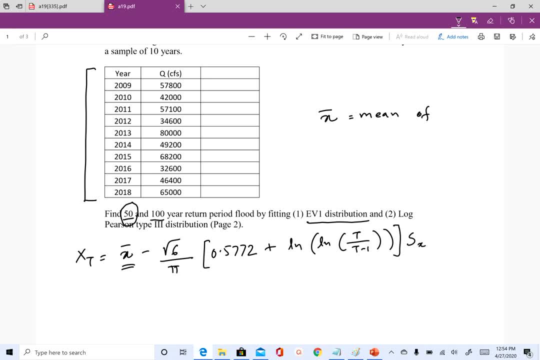 mean of sample, which will be the mean of our Q annual maximum series, and Sx is the standard deviation of sample. Okay, and t is the return period. Okay. so instead of Xt I'm just going to say Qt here. X bar you can get the mean of. 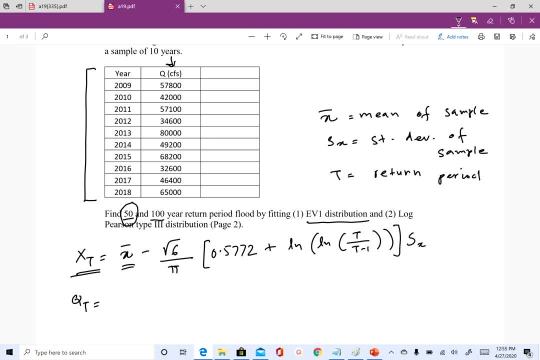 this series, if your calculator allows you to do that. if not, what you can do is so: X bar is Q bar is equal to summation of all Q's divided by n, So n in this case is 10.. Okay, so n is 10.. I have done these calculations for you, so for this we. 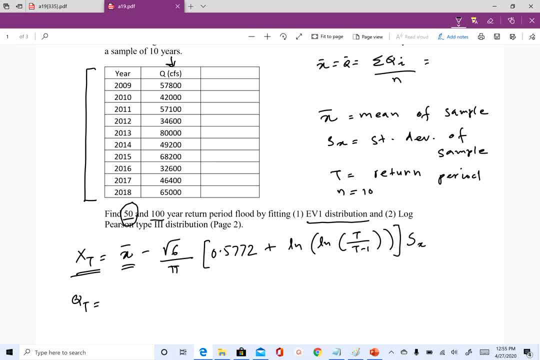 have mean of 53,290 CFS and then for standard deviation, either you can use your calculator if your calculator does not allow to calculate standard deviation. So the expression that we have for standard deviation is 1 over n minus 1.. So X minus. 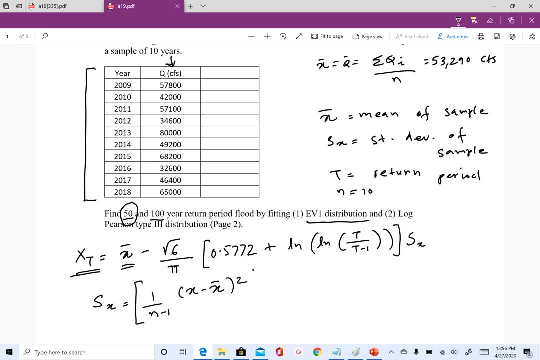 X bar square, And then you take the square root of that. So again, X in this case is all our discharge values and X bar is the mean discharge, which is 53,290, and again I have done this for you, so the number that I got is 15,190 CFS. Okay. so once you have these two numbers, so Sx will be this. 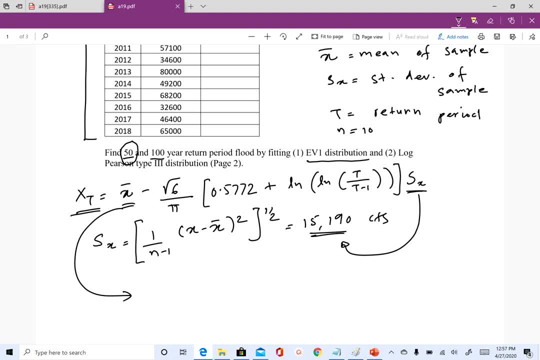 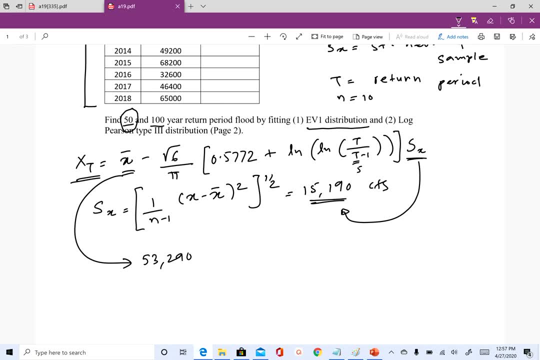 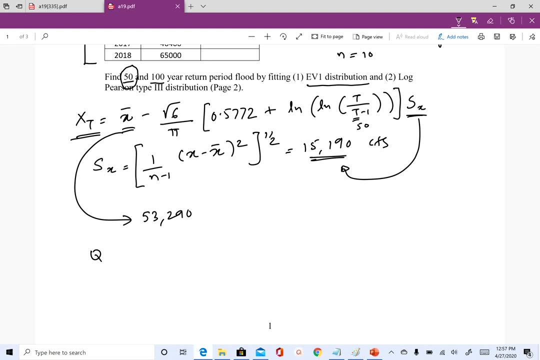 And X bar will be 53,290.. t is 50 for the first return period, so Q 50 is going to be 53,290, minus square root of 6, divided by PI 3.142, 0.5772 plus. so this is natural log just. 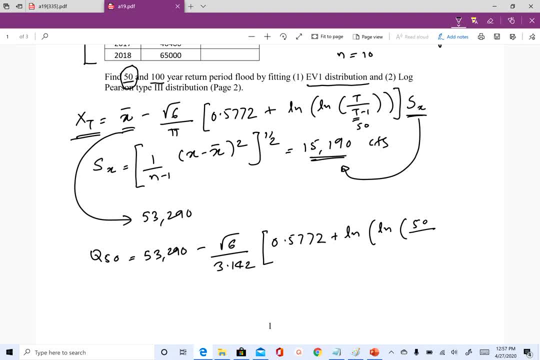 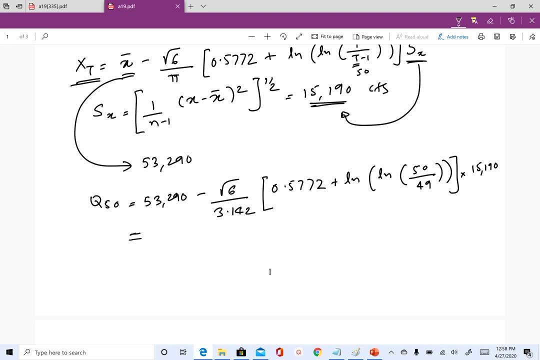 remember that. so T is 50, and 50 minus 1 is 49, and then you multiply this whole thing, this part, by 15,190. so you do all this and the answer that I got was 92,663, and you really don't need to worry about the decimal places here. so I 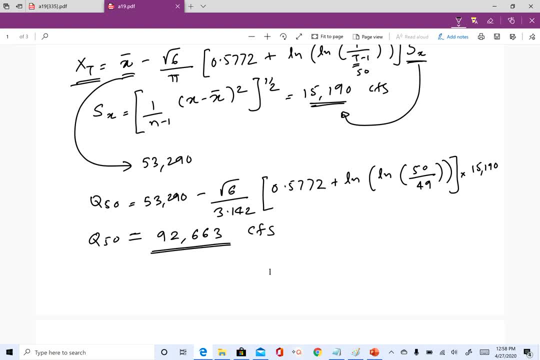 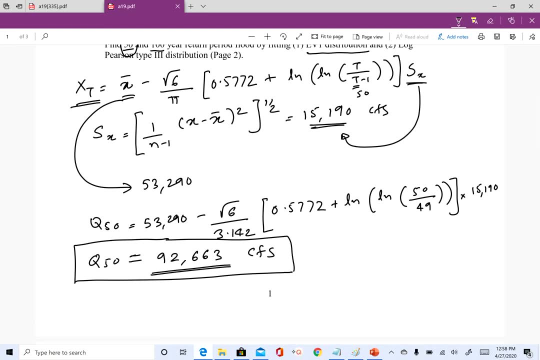 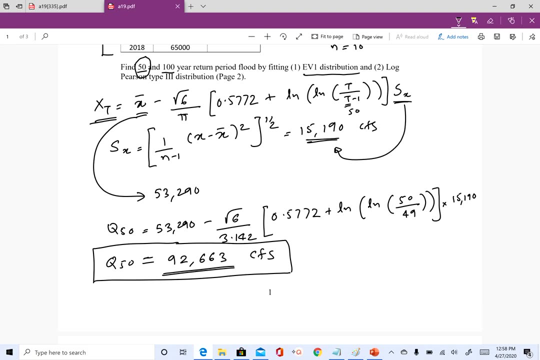 have rounded it out up the number, so CFS. okay, so you can see this is a relatively straightforward method. if you are going to use ev1 distribution, or if you assume that the data fits the ev1 distribution, okay, and figuring out which distribution fits is 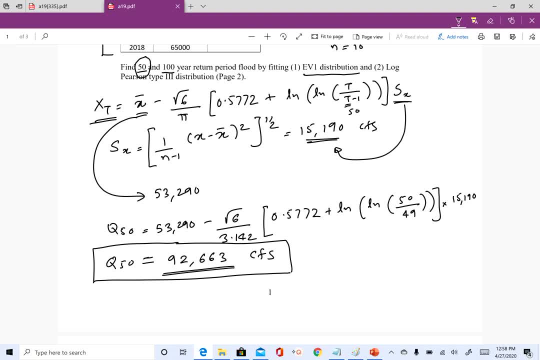 a whole different topic. so in this case we just assume that we are going to use ev1 distribution for question number one. okay, so I have done this for Q 50, you, I want you to do this for Q 100. so the only thing that will change in this 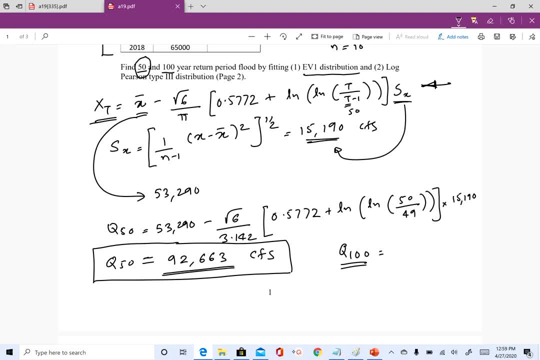 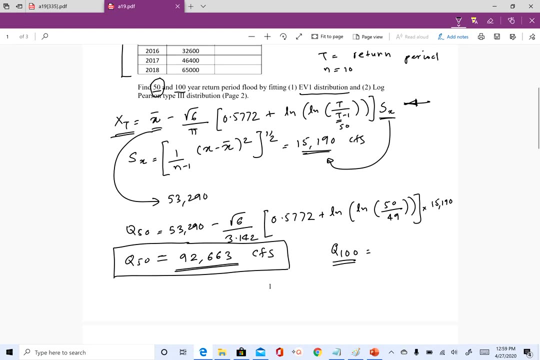 expression. when you are doing this for Q, 100 will be T. so in this calculation, I use T equal to 50. when you do this for Q 100, I want you to use T equal to 100, and that's as straightforward as it is. the other thing i want you to see from this is that when we did 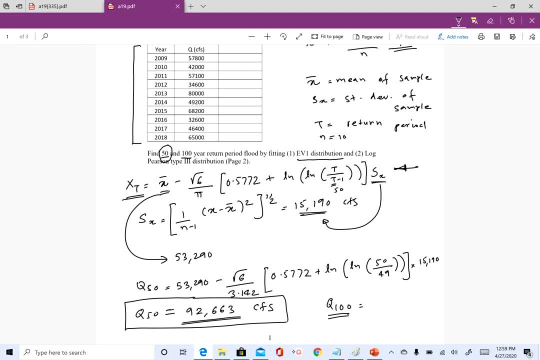 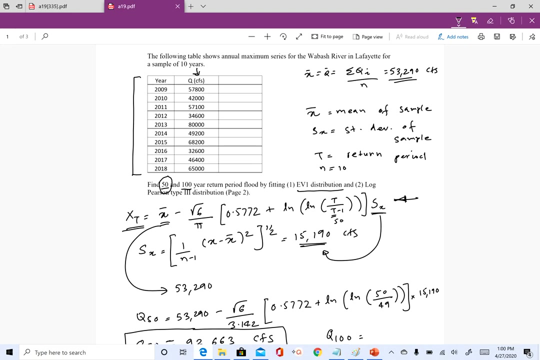 the exceedance probability approach. in the last assignment, you can see that the number that we got is different than what is included in the sample. so that's the advantage of using the probability distribution function. okay, so this is how you can do flood frequency analysis using ev1 distribution. i gave you an empty column here, just in case if you want to use the 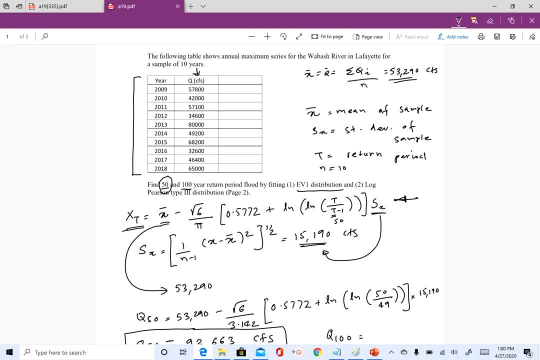 empty column to get the values for calculating the standard deviation. so in this case i can just use this column for x minus x bar and write down all these values and get the sum here and use that sum in this expression. so if your calculator allows you to, 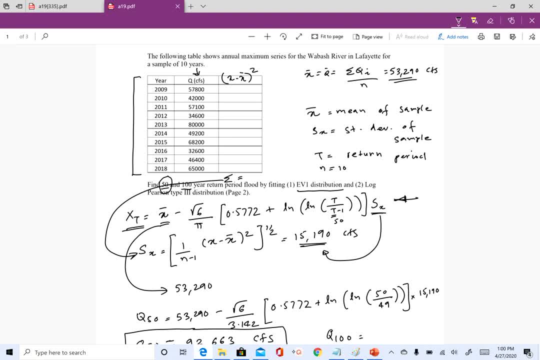 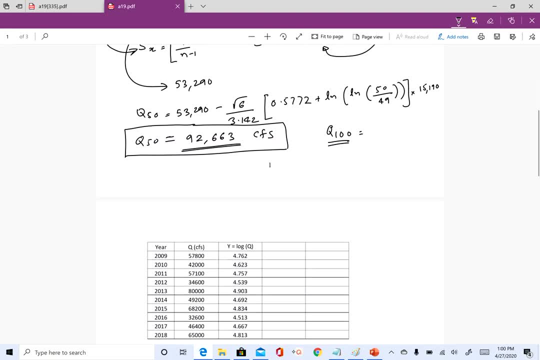 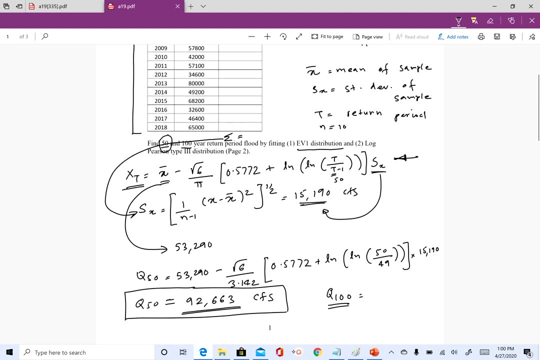 do the standard deviation calculation, you don't need this column, but if not you can use it. so so this is how you can do flood frequency analysis using ev1 distribution. so in the next question i asked you to do the same using log pearson type 3. okay, 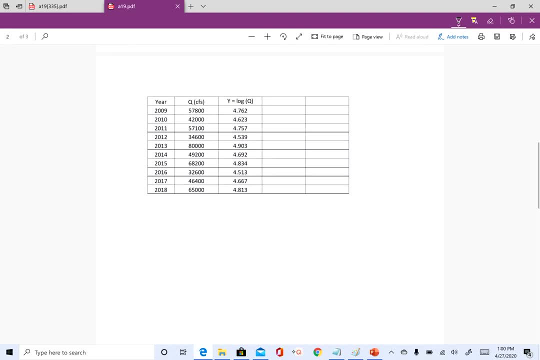 so this is on page 2 of your assignment. so the the method that we are going to use for log pearson type 3 is the frequency factor method. so the frequency factor method says you first have to find y t, so which is y bar plus k t times s, y, and once you get y t, then x t or q t will be 10 to. 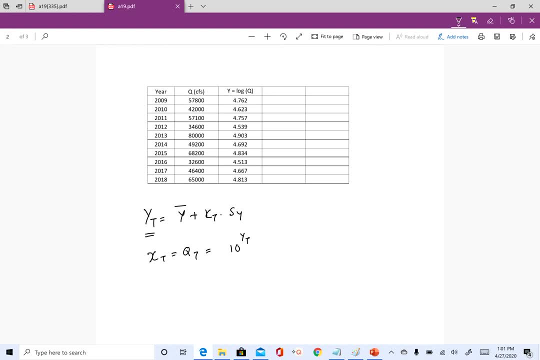 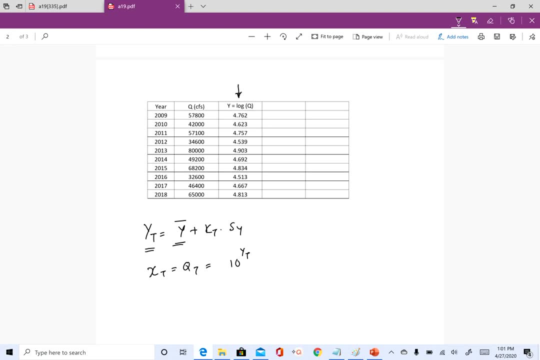 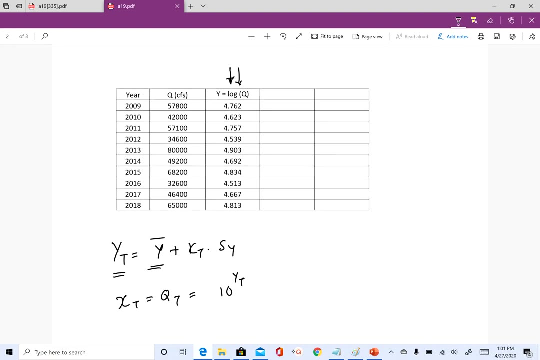 YT, okay. so to do this we need the Y series. so Y series in this case is log of Q, okay. so again, I have done this for you. you can verify the numbers that I got and I hope you are able to see these numbers. so I have created the Y series. 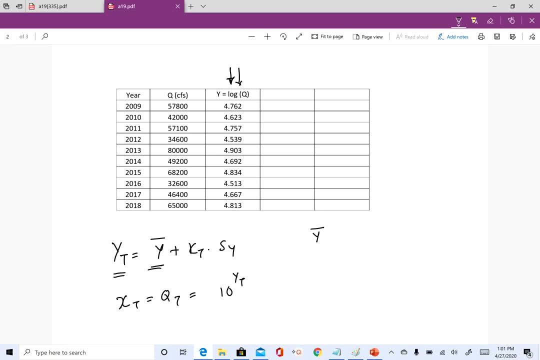 for you. so once you have the Y series, you get Y bar and S Y, similar to what we did before for the Q series. so again, this column: if you want, you can use this as Y minus Y bar square and you get the sum. and you calculate the sum by: 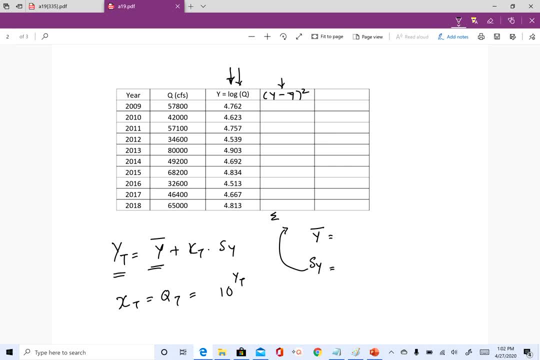 standard deviation by using this sum. so again, I have done this for you. so Y bar that I got is four point seven. one CFS and S Y is zero point seven. one CFS and S Y is zero point seven. one CFS and S Y is zero point. 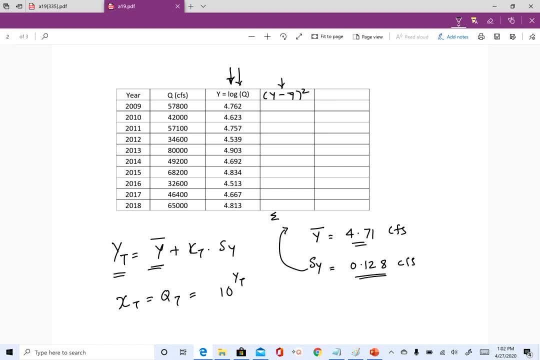 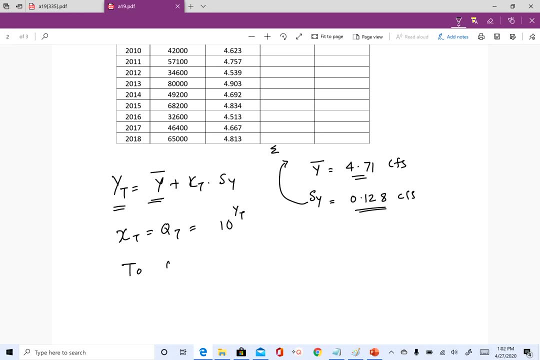 one, two, eight, CFS, okay, and then we have to find KT. so to find KT, you need to know, to find KT, we need to know coefficient of skewness and T. so T is 50 for this and the expression that we have for coefficient of skewness, which is 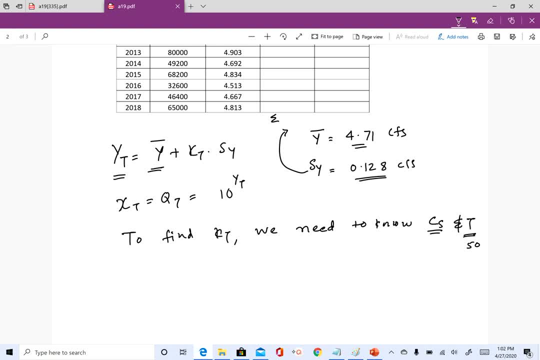 in the powerpoint that I have given you in the last video, but I will still write the expression here, which is n, summation of, so this will be n X I minus X bar cube, so summation of all the cubes of these differences. so I is equal to one. 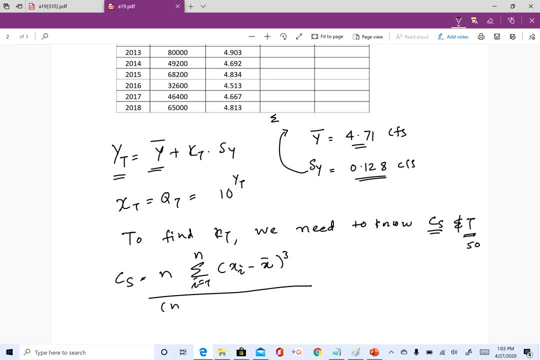 to n and divided by n minus 1, n minus 2 times S cube, so X bar is, in this case, we are doing this for Y series, so Y bar and S cube is S Y cube, okay, and n, in our case, is 10. so you have all that you need to get the 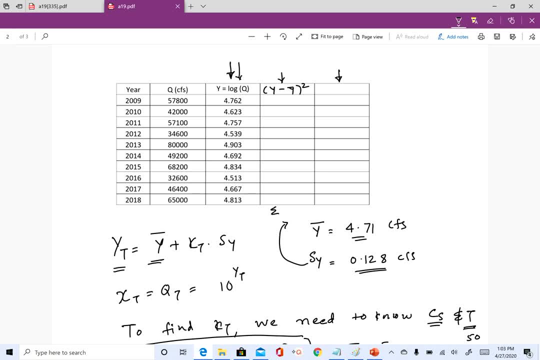 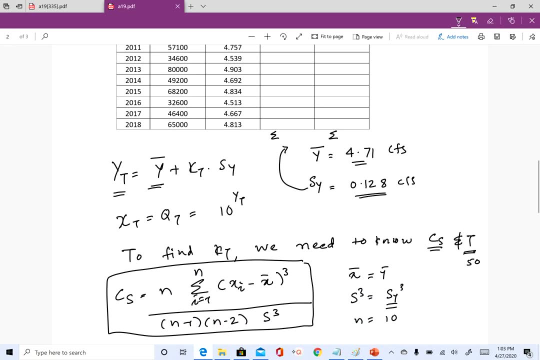 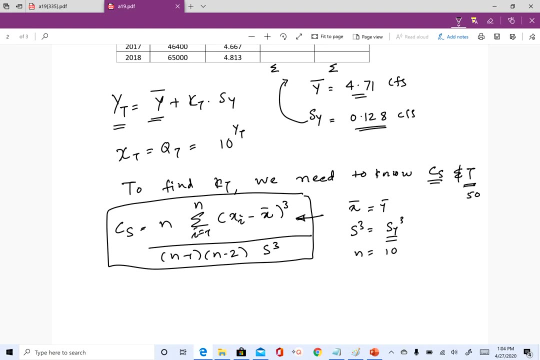 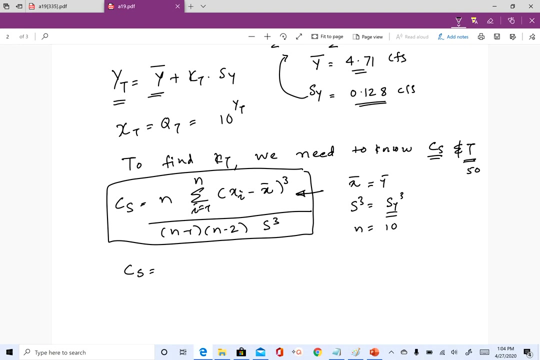 coefficient of skewness. if you want, you can use this column to get Y minus Y bar cube and sum those values and put that sum here to calculate the coefficient of skewness. so again, I have done this for you. so C, Y instead of yes. so CS or coefficient of skewness, CS of. 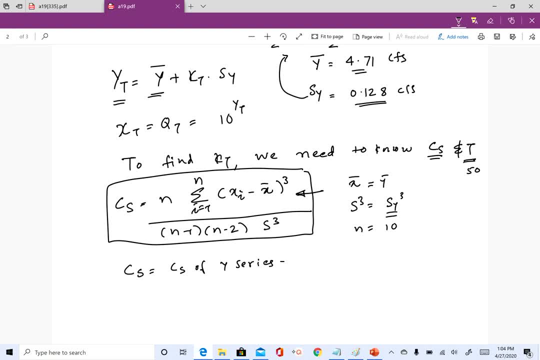 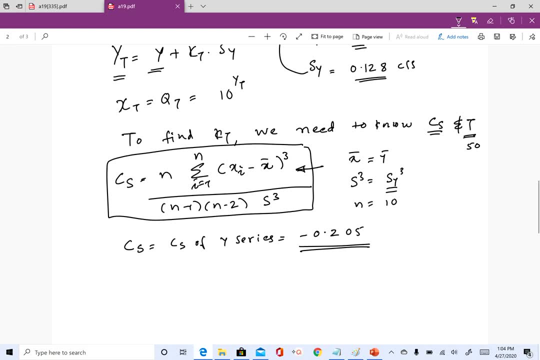 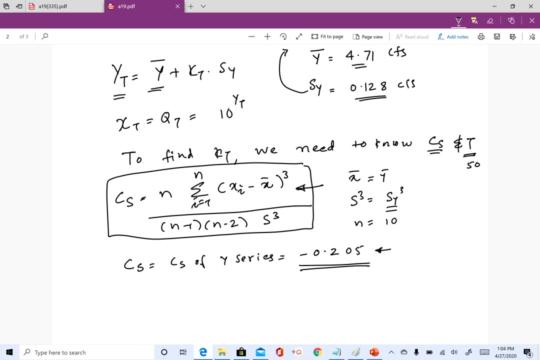 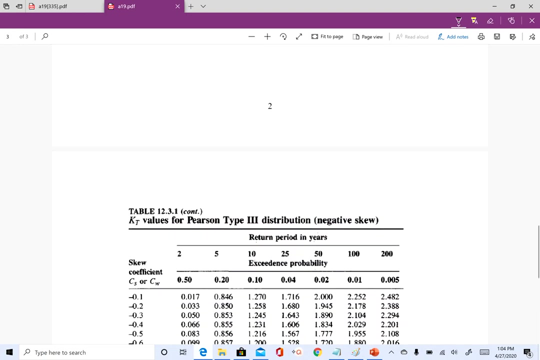 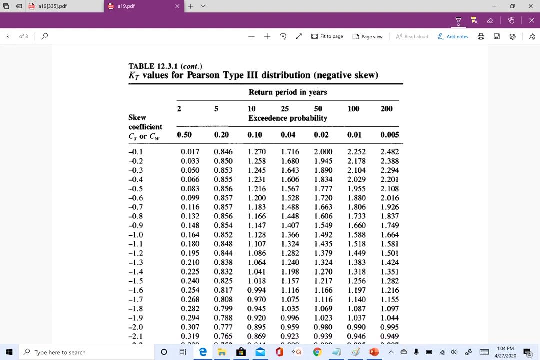 Y series that I got was minus zero point two zero five. okay, so once we know what the coefficient of skewness is, once we know what the T is, we can use the table that I showed you in my video, and I have also given you the table in this assignment. so this is the assignment page that you can use. so 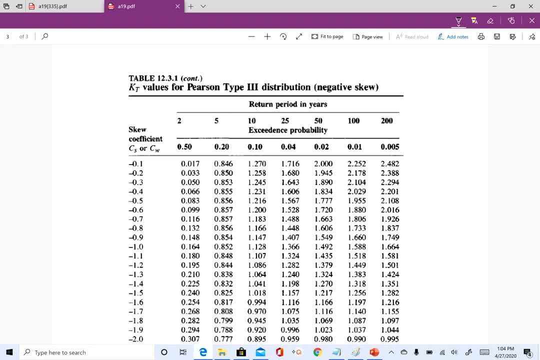 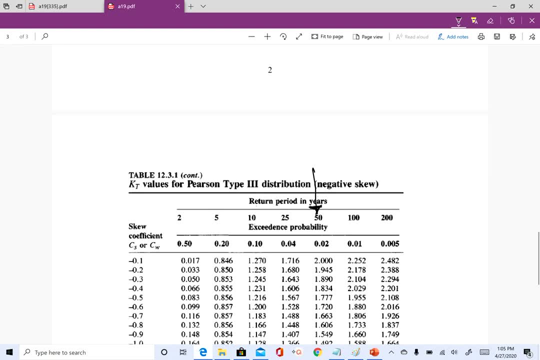 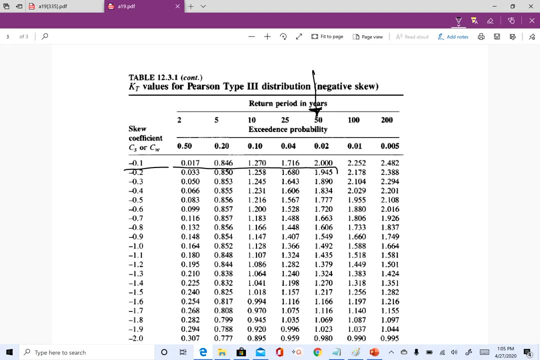 we are looking at the table that you can use in this assignment and in this at return period of 50, so I'm going to look into this column and our coefficient of skewness is 0.205, negative 0.205, so our coefficient of 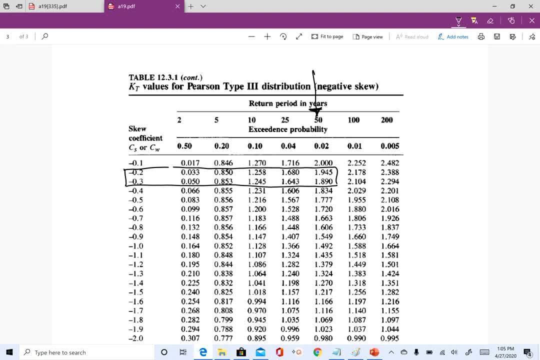 skewness is going to lie somewhere in between these two values, which is 1.945 and 1.890. so for negative point to its point, it's 1.945 and our coefficient of skewness is 0.205. so it is going to be very close to 1.945. so I'm just going to 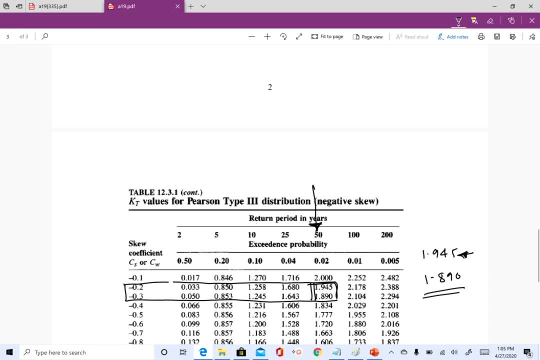 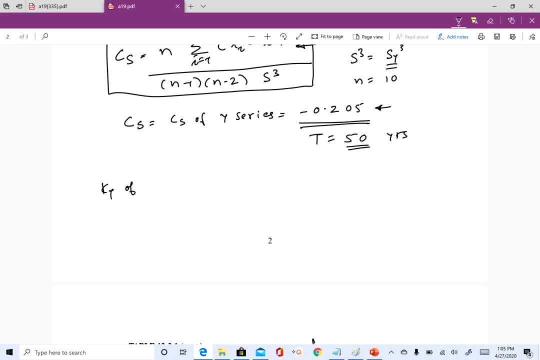 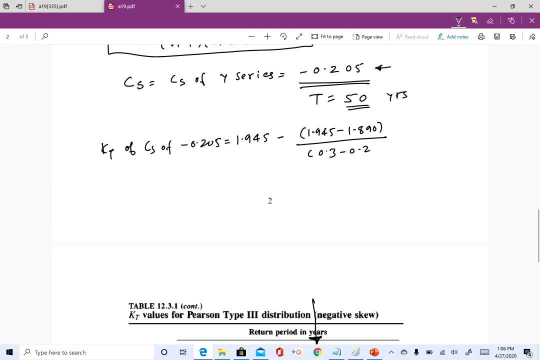 linearly interpolate that, so I will use point one, point nine, four, five and one point eight nine zero. so KT for CS of minus 0.205 is going to be so 1.945. I'm linearly interpolating it, so this is the value for 0.2. so 1.945 minus 1.890 divided by 0.3 minus 0.2. yeah, 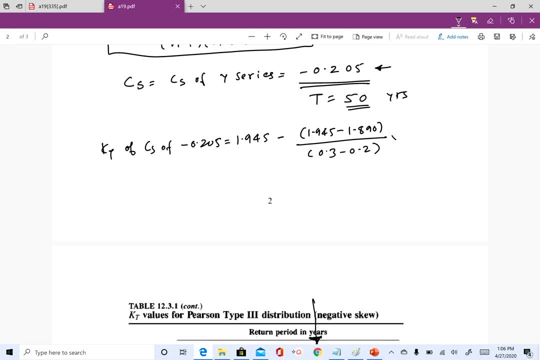 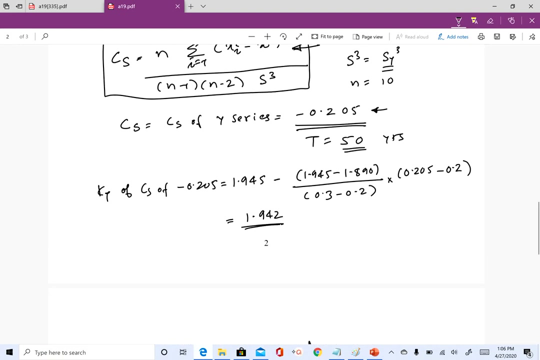 and then we do 0.205 minus 0.2. okay, so once you do that, the value that I got was 1.942. so we will use three decimals. so depending on how many decimals you use, the answer may be slightly different. so once we get kT, then we can find YT, so YT. 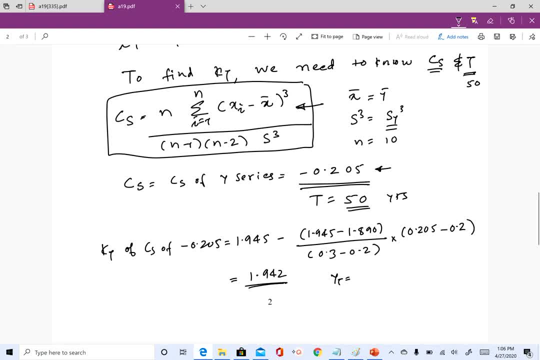 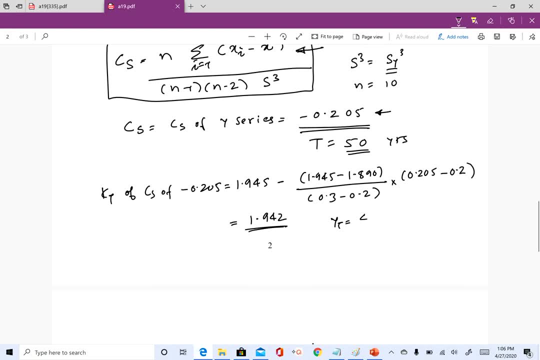 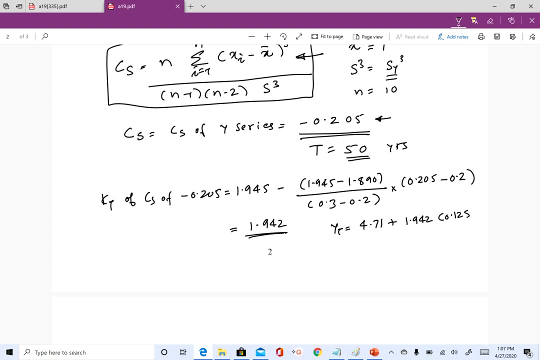 is going to be y by t, Let's do it right now Yt. so y bar in our case is 4.71 plus kt times sy. so kt is 1.942 and sy is 0.128, 1.128, and once i solve that, the value that i get is again up to three decimals. 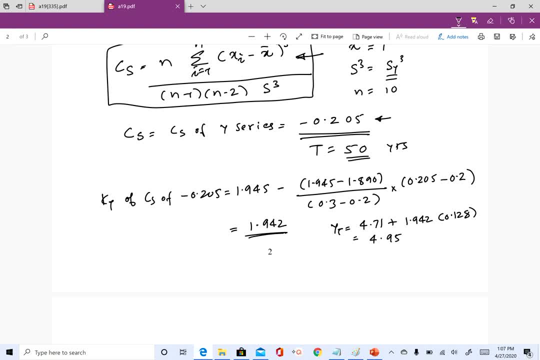 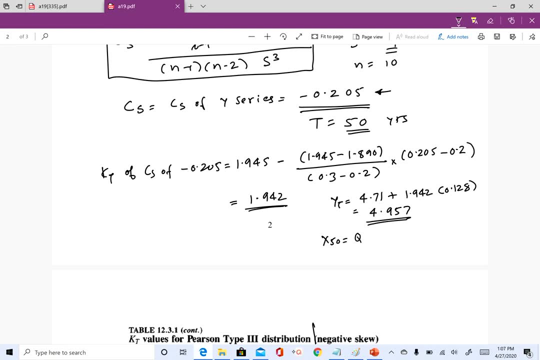 4.957, and once i have that, my xt, so x50, which is q50, is 10 to the power of 4.957. and then, if i solve that, the value of 4.957 is 10 to the power of 4.957. 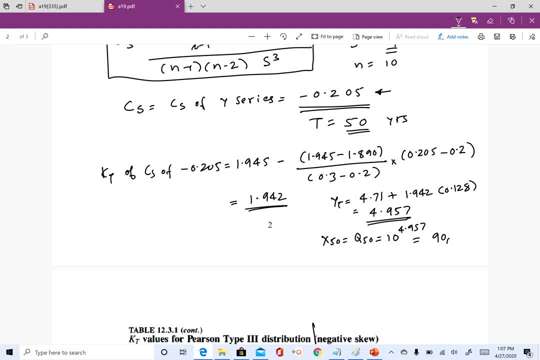 and then if i solve that, the value of 4.957 is 10 to the power of 4.957 that i got was 90 570 cfs. okay, so this is the answer that we have for 50 air flow. i'll just. 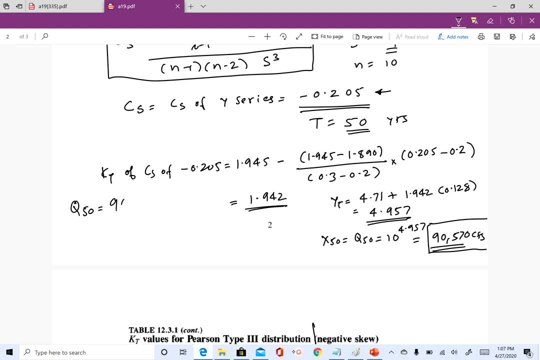 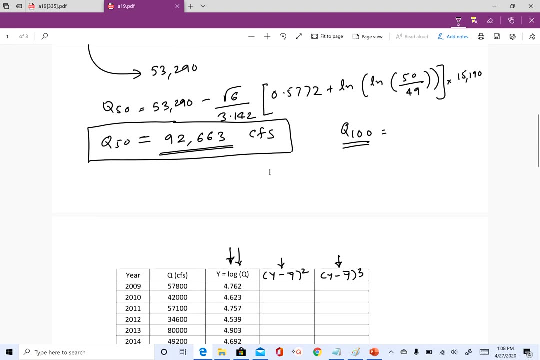 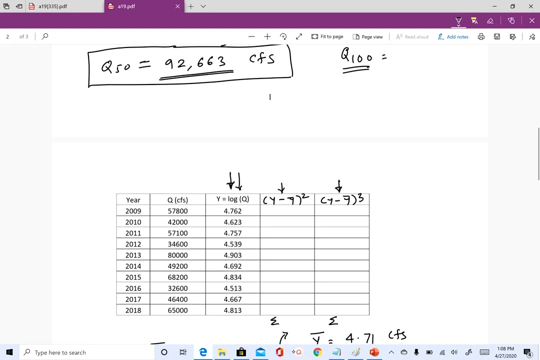 write down that here. so q50 is 90 570 cfs. so this is using lp3. if i go back and look at the answer that i got, that i got for ev1, which is 92663, so you can see that these numbers are slightly different. 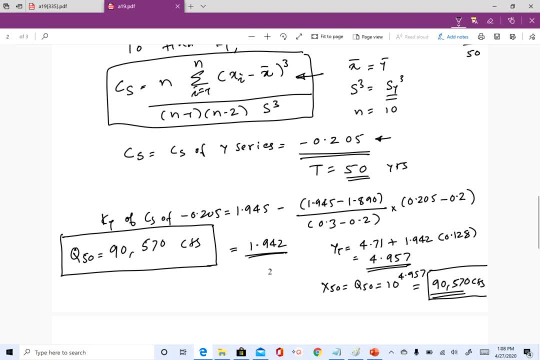 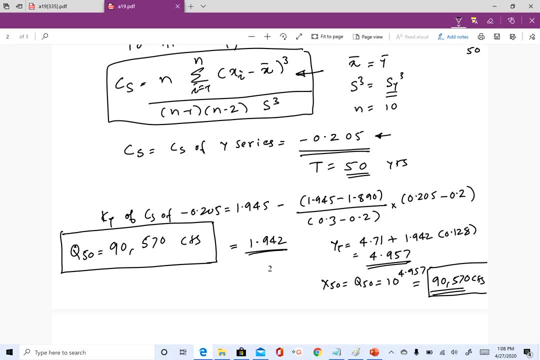 but they are not too far off from each other. okay, so this is how you can use the log pearson type 3 method to get the flow corresponding to return period. so now i did this for you, i want you to do this for also 100 year flow. so the only way to get the flow corresponding to return period. 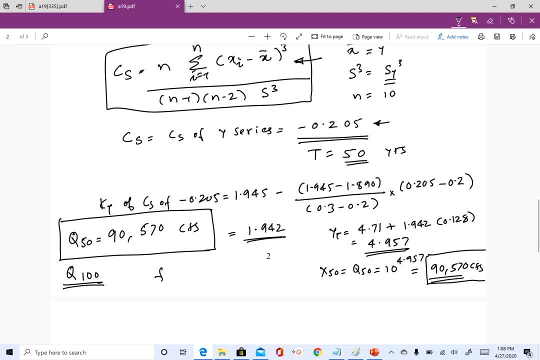 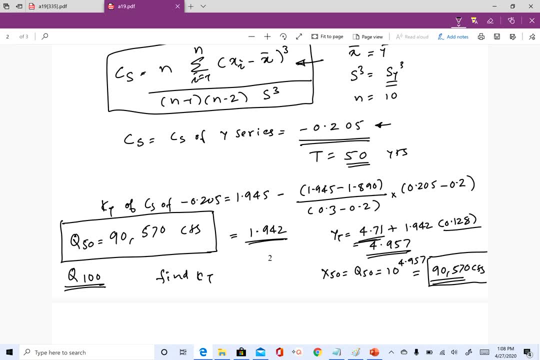 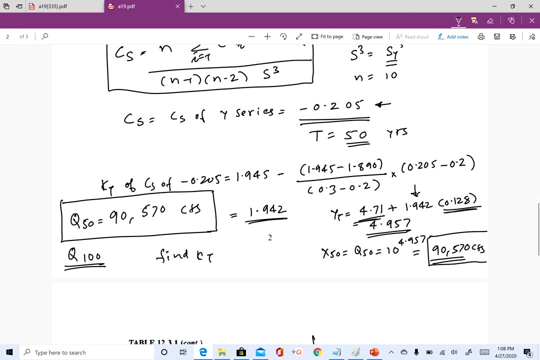 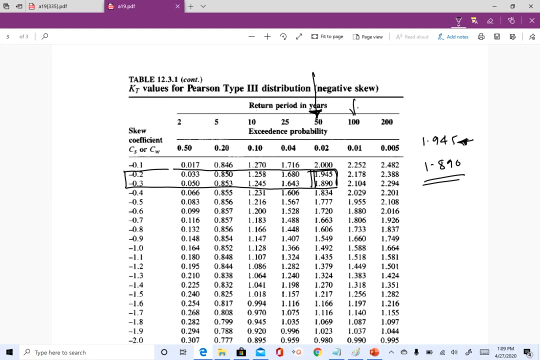 the only thing that you need to do in this case is find kt. once you get kt, y bar will not change. sy will not change. all you have to do is replace 1.942 with what you get for the 100 year flow, so again you can use the same table. so in this case we are looking at this column for 100 year flow and our coefficient.